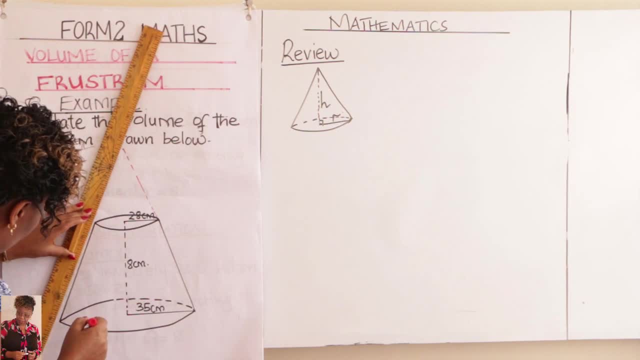 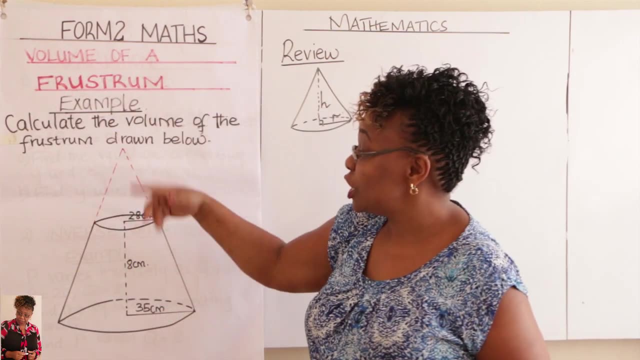 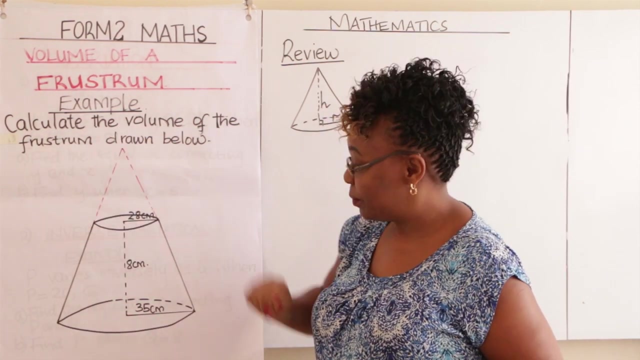 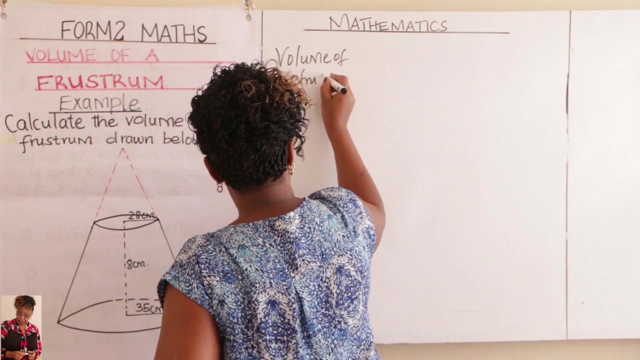 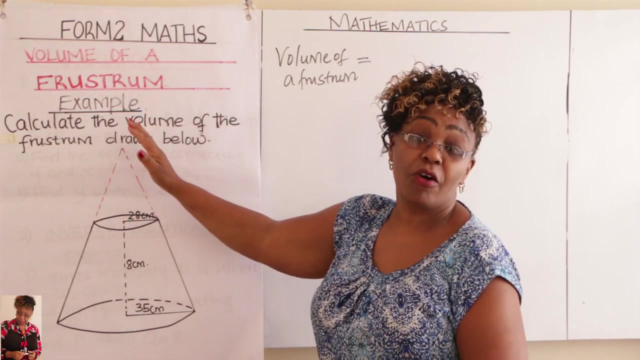 them. with a ruler like that, We also produce this other one like that, so that we get the original cone from which the frustrant was obtained. So this is now the original cone: Volume of a frustrant learner. Volume of a frustrant learner is got by finding the volume of the original cone and then you subtract the. 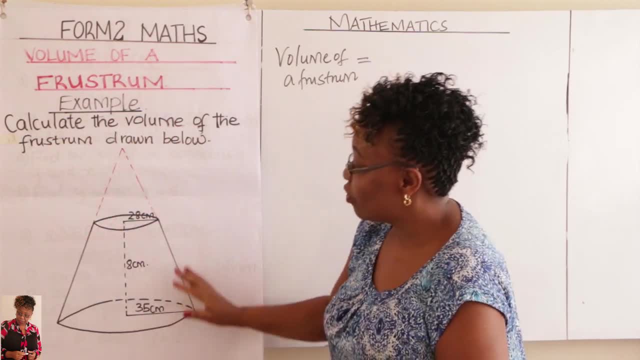 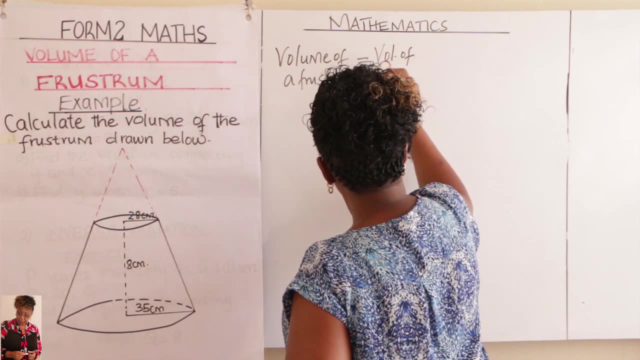 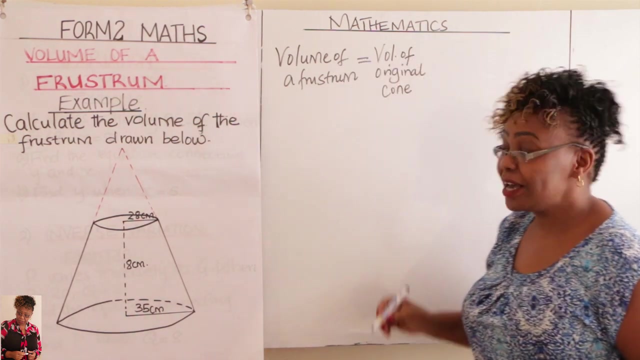 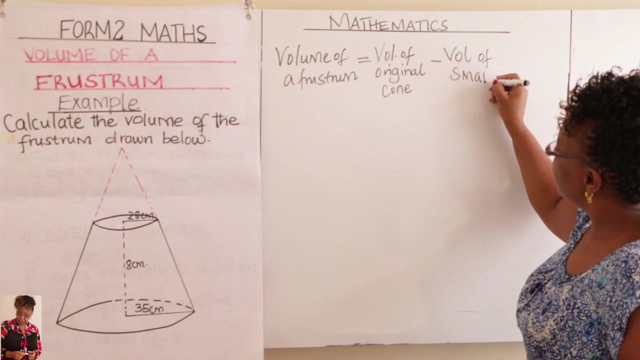 volume of the smaller cone. Volume of the original cone minus volume of the smaller cone. So this is: volume of the original cone, volume of the original cone, yes, minus volume of the small cone, minus volume of the small cone. so learn. volume of the. 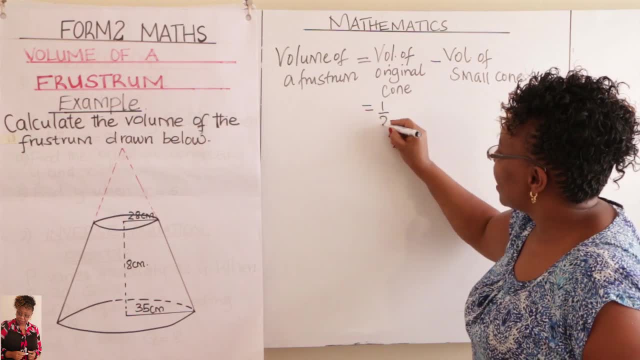 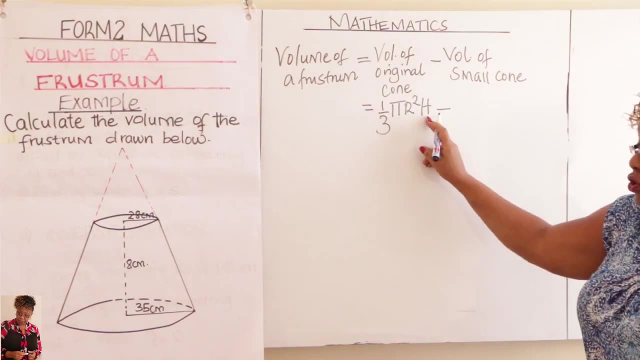 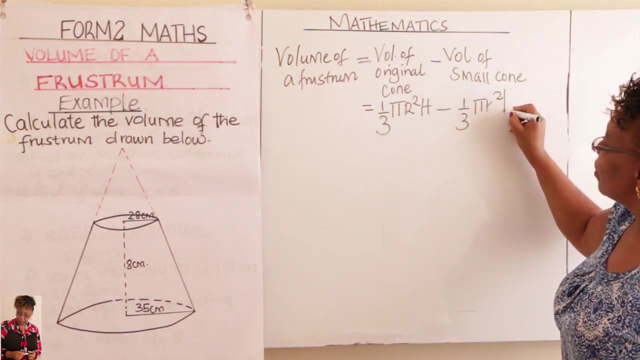 original cone will be obtained using a third pi r squared height. we use capital letters for r and h because we are talking about the big cone. then you subtract the volume of the small cone of the small cone. yes, so you look at our formula here. what do we have? 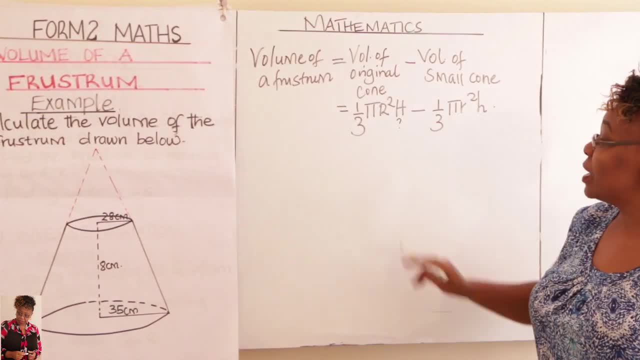 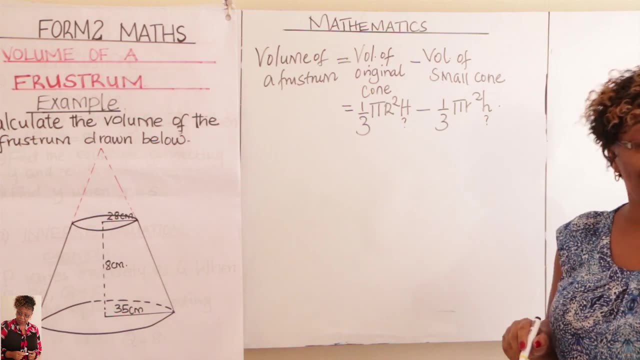 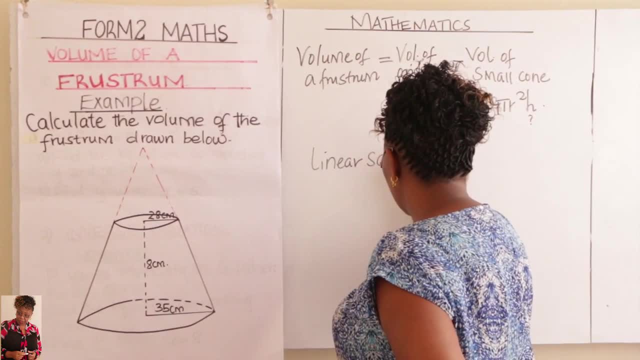 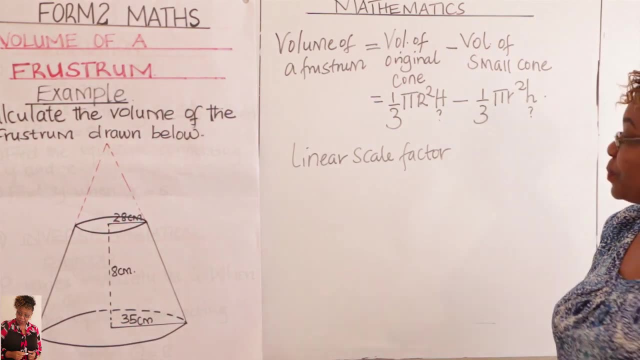 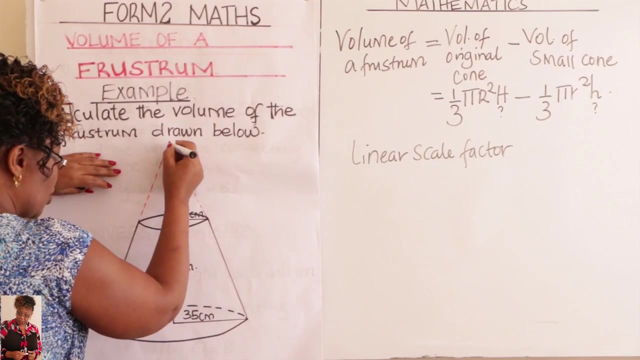 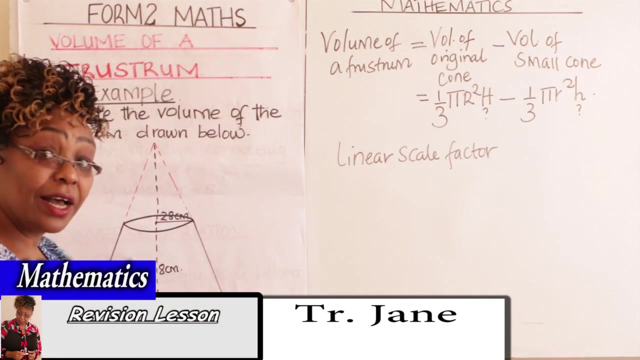 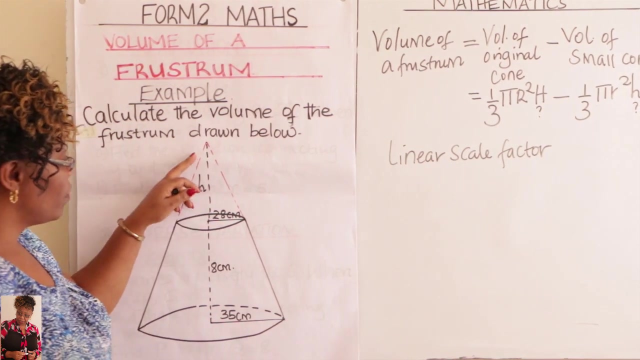 okay, okay, okay, to get h linear scale factor, you use linear scale factor, similar triangles, that is. so you come here and you introduce your height, the small height. come here and you introduce your small height. call it small h there. so, using linear scale factor, we talk of small h. 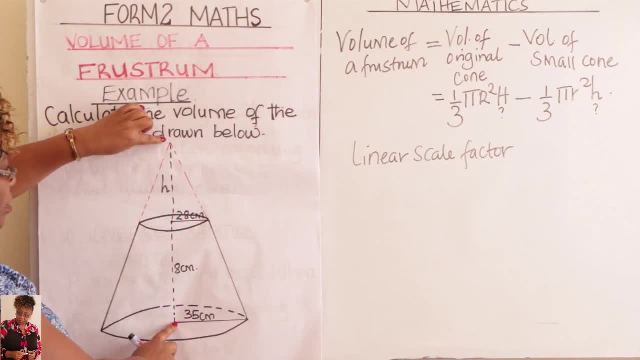 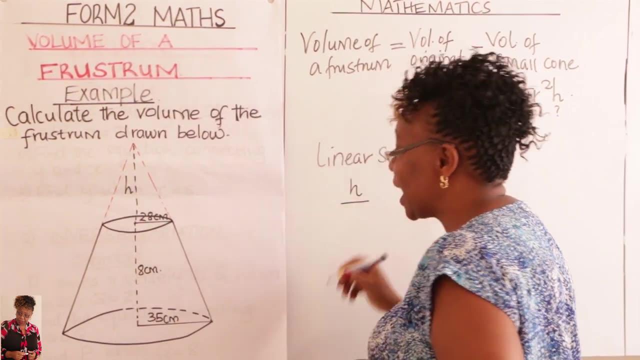 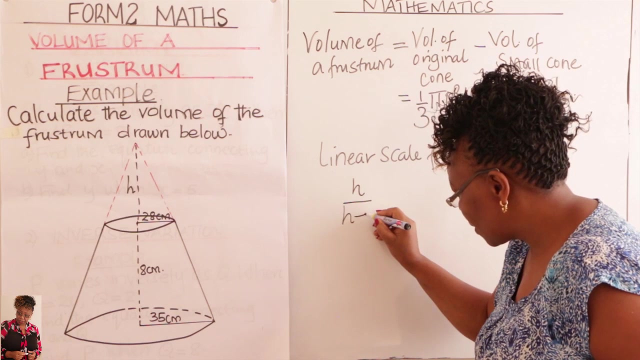 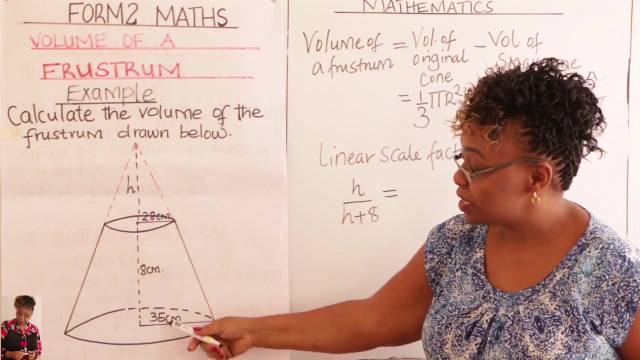 small h over capital h. this is your capital h from here to here. so we talk of small h over capital h, which is h plus 8. h plus 8 is equals to what which are the two corresponding signs. they will be 28 over 35. 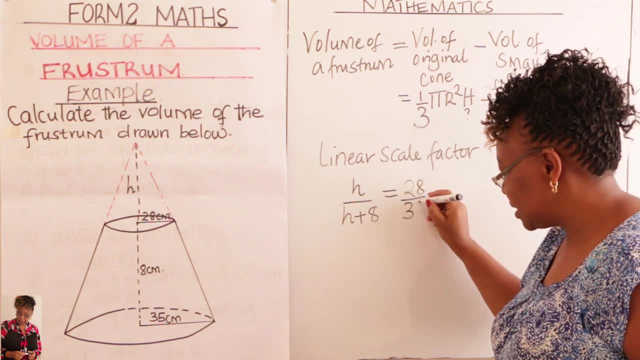 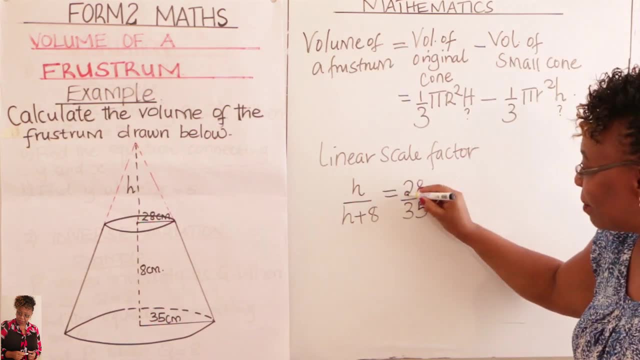 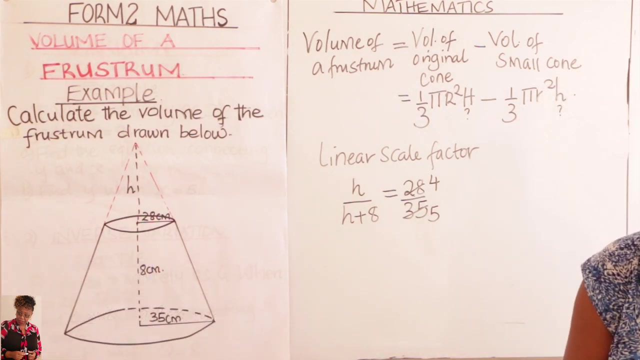 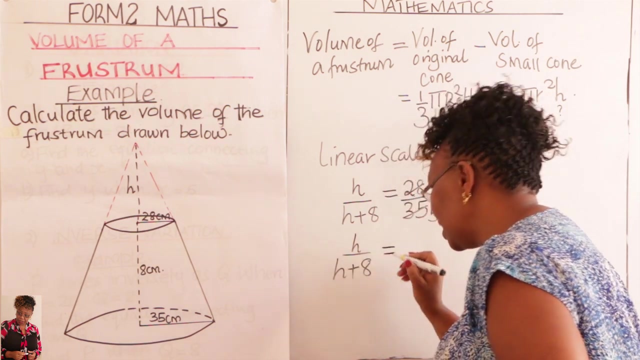 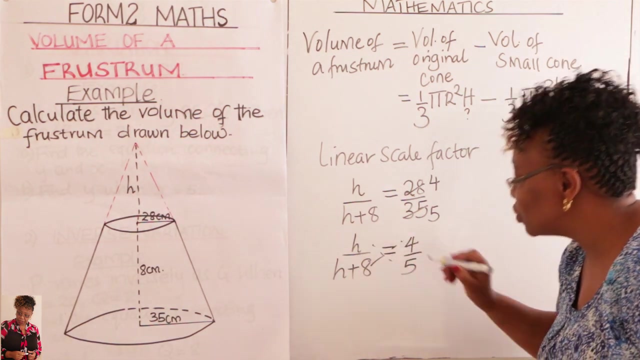 28 over 35. work out this line by 7, 4 by 7, 5. you simplify so small h over h plus 8 should therefore give you 4 over 5. yes, cross multiply, cross multiply this. this will give you 5h. 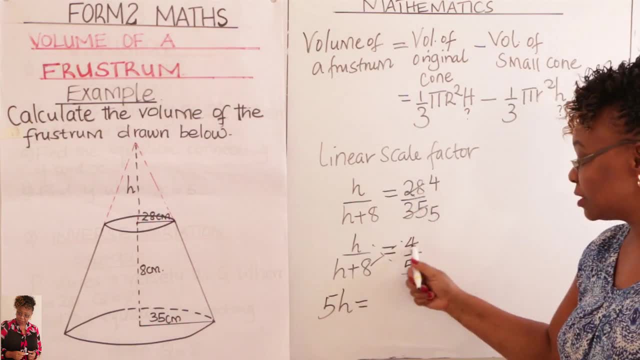 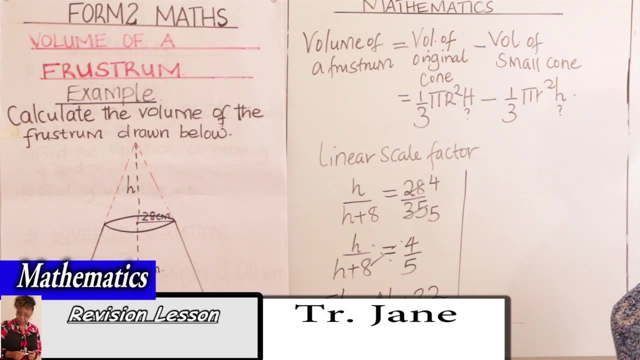 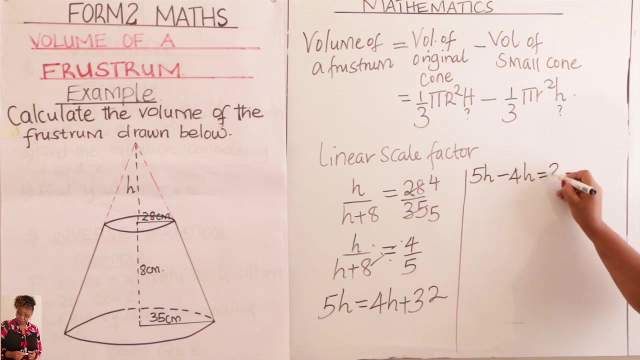 is equals to what? multiply this by 4? multiply this by 4 gives you 4h plus 32, 4h plus 32. so you take this to the other side, you get 5h minus 4h is equals to 32 and therefore you subtract this. 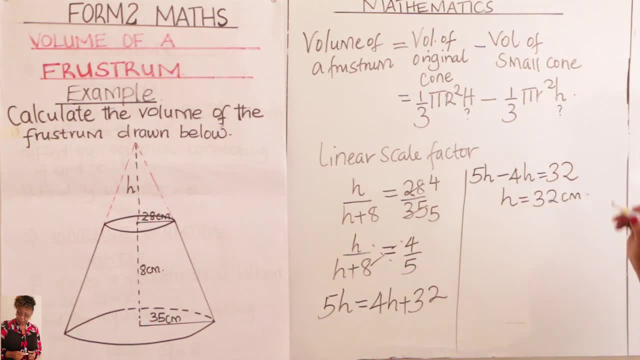 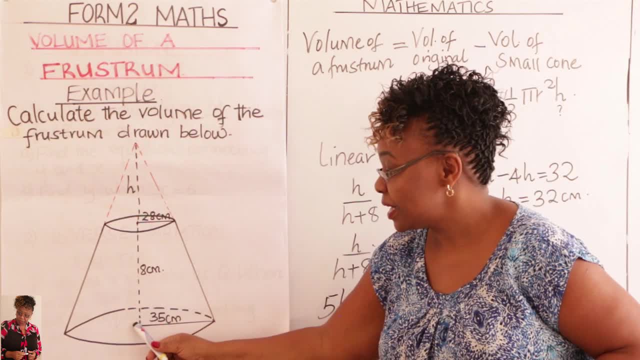 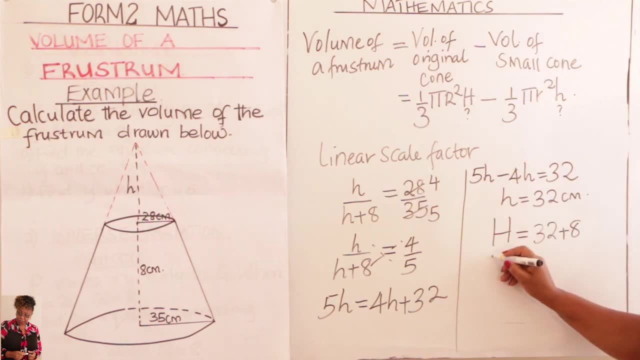 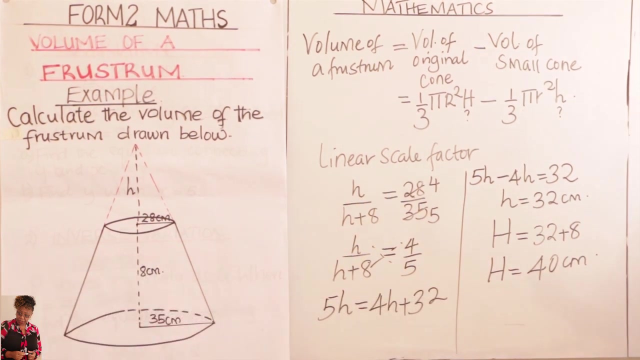 which you have already got as 32 plus 8 small h, which is 32 plus 8 small h plus 8. so your capital h is 40 centimeters. yes, from there now we now go to the volume of the capital h, which is the volume of our first round. 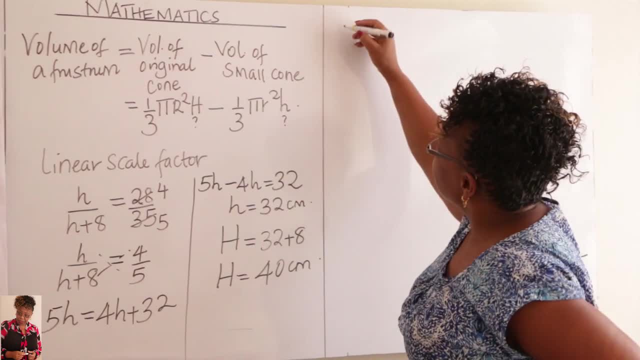 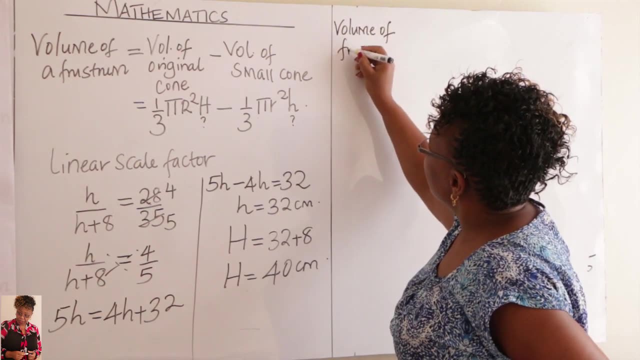 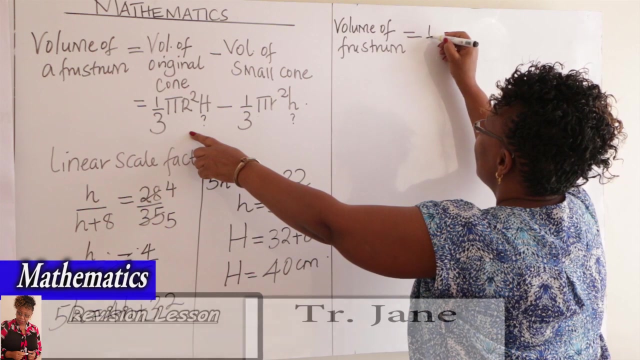 so how do we get the volume of our first round? so we come and say: the volume of our first round, the volume of our first round, the volume of our first round is therefore equal to what you come to your formula a third times 22 over 7.